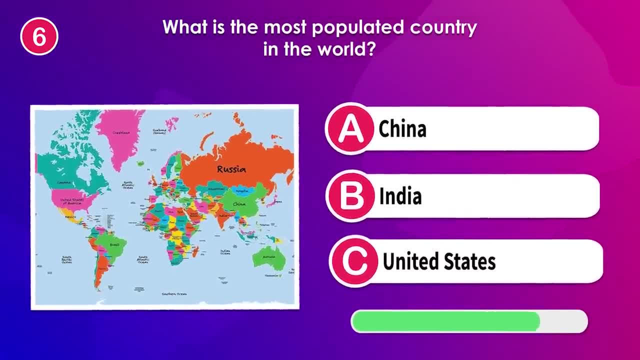 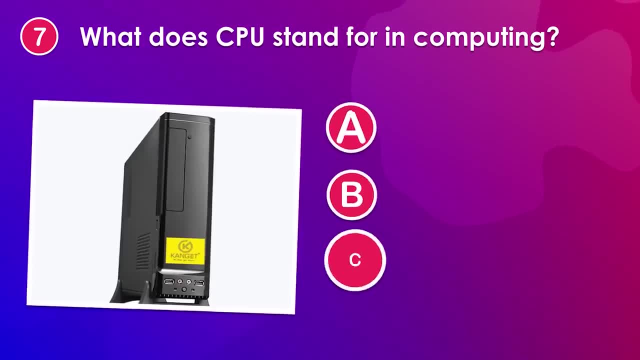 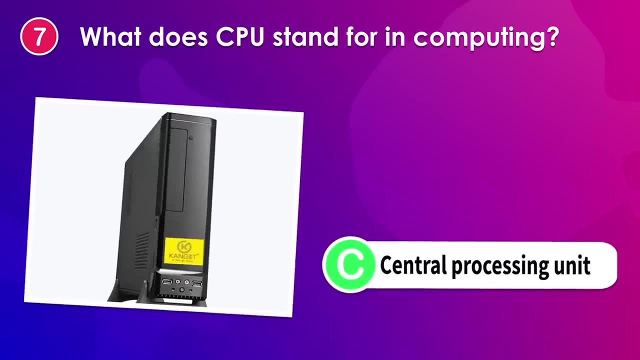 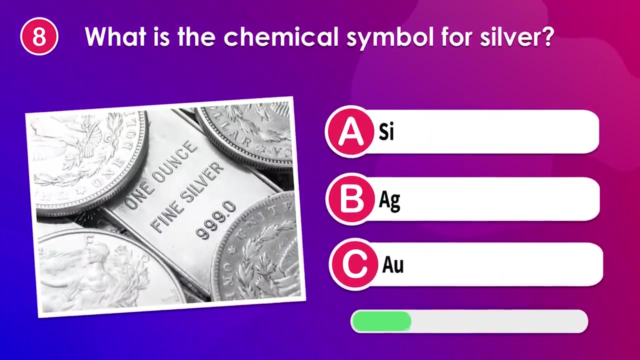 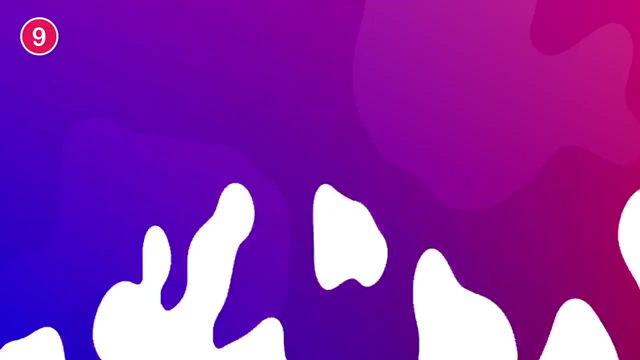 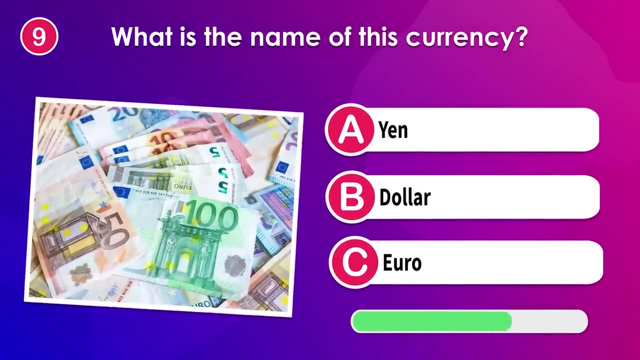 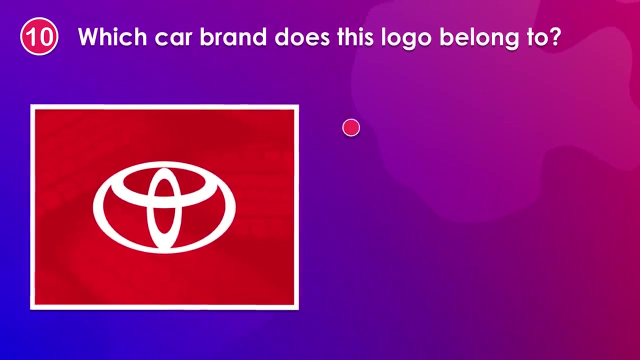 The answer is Brazil. We're very good at results. What does CPU stand for? The correct answer is the central processing unit. What is the chemical symbol for silver? What is the name of this currency? It's Euro. Which car brand does this logo belong to? 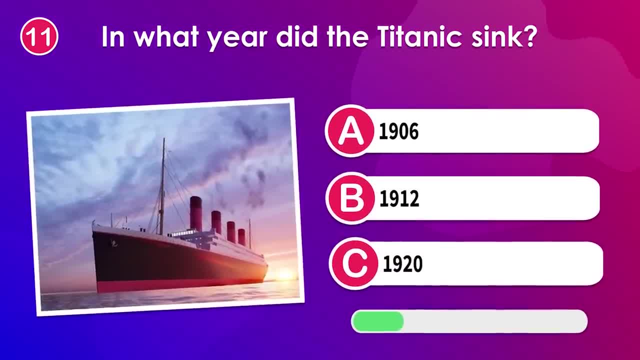 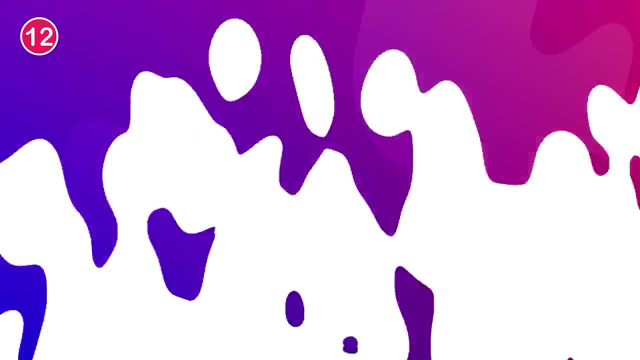 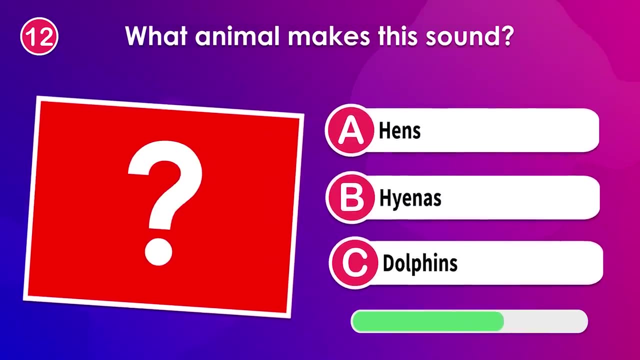 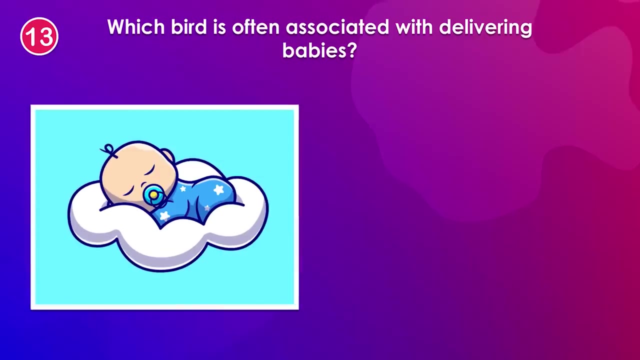 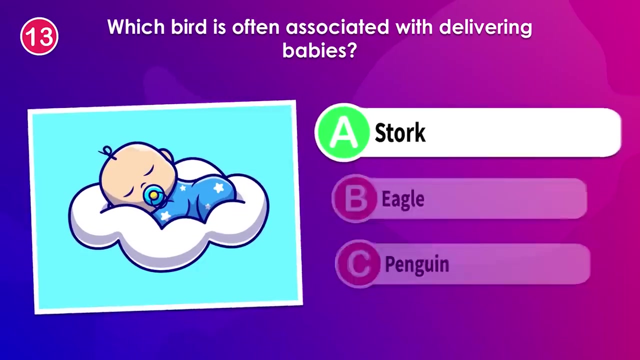 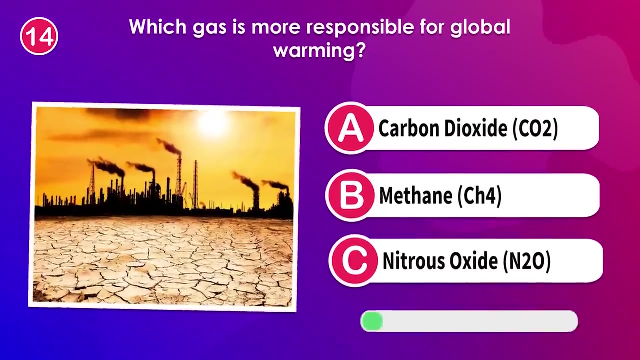 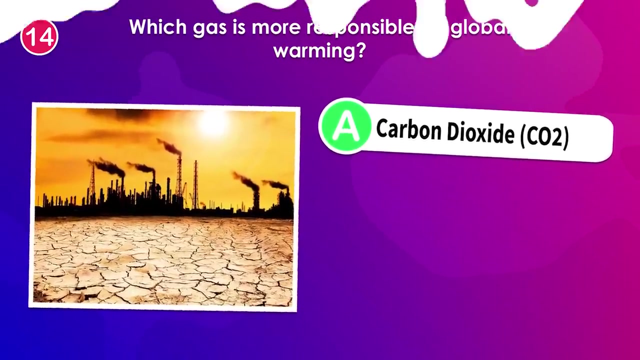 In what year did the Titanic sink? It was 1912.. What animal makes this sound? The correct answer is dolphins. Which bird is often associated with delivering babies? Which gas is more powerful? Which gas is more responsible for global warming? Carbon dioxide is the right answer. 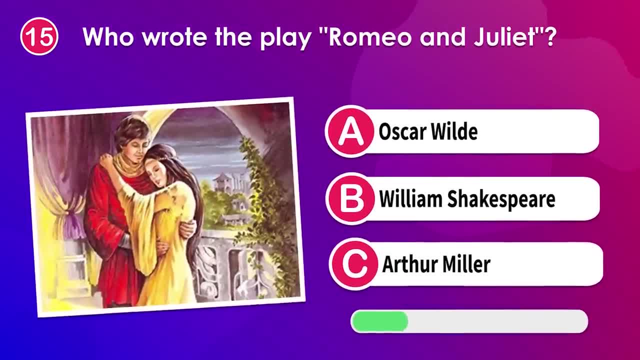 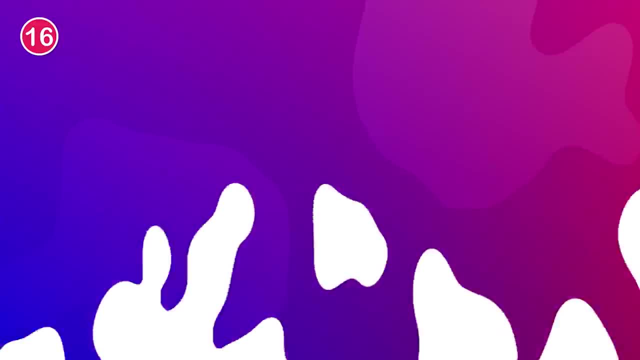 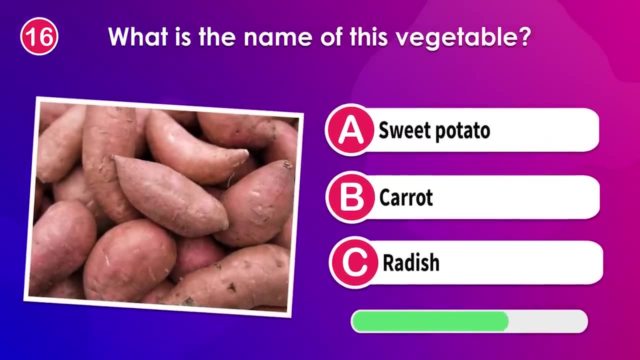 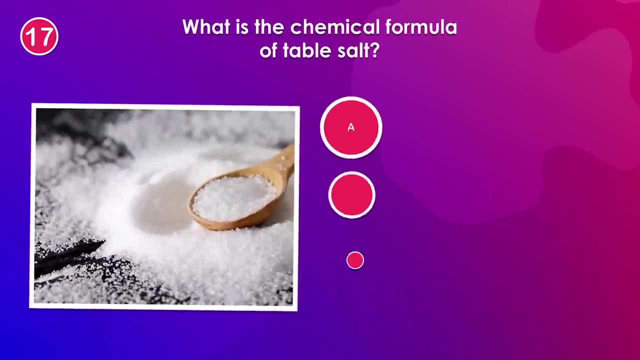 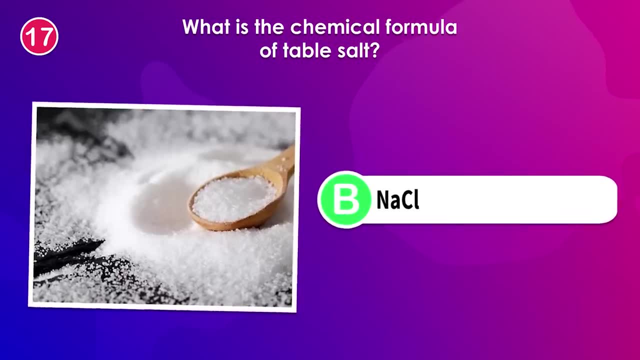 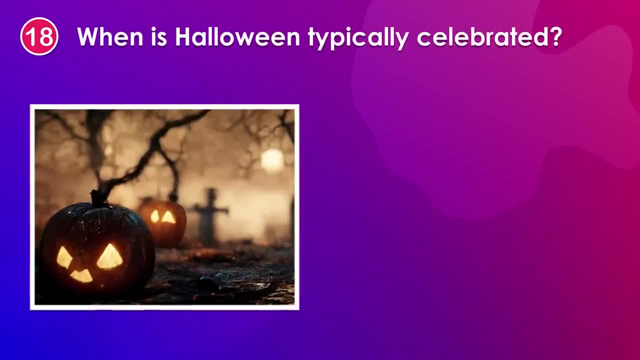 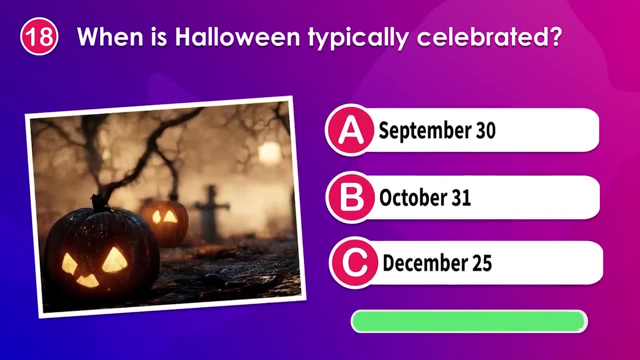 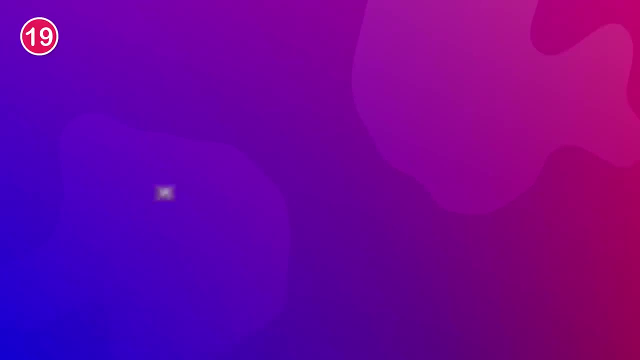 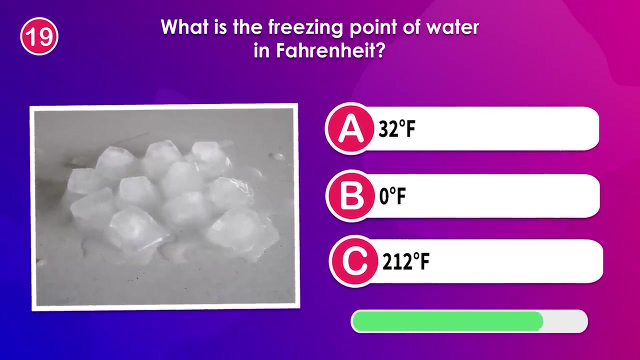 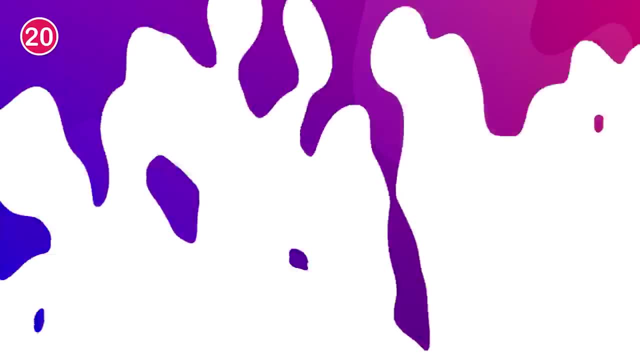 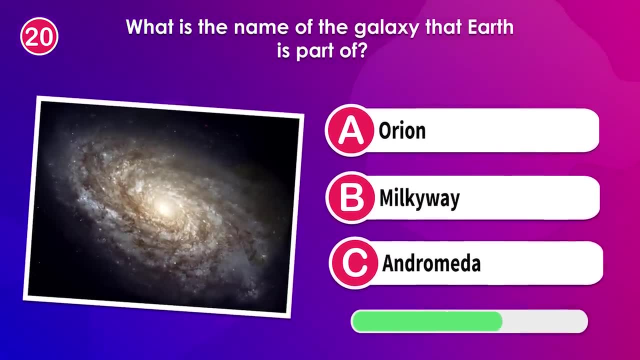 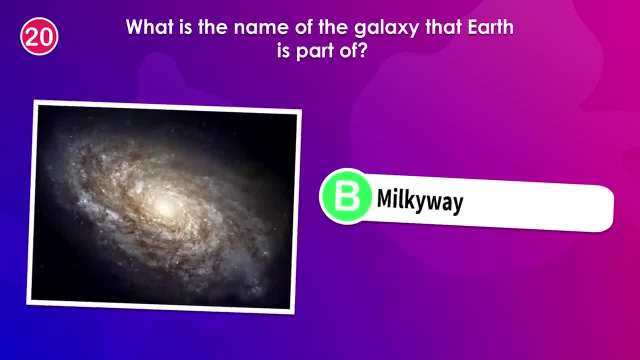 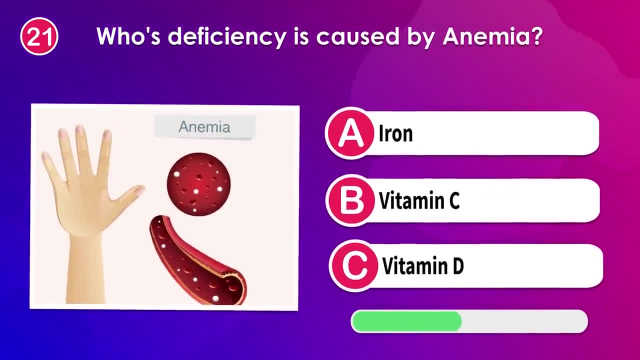 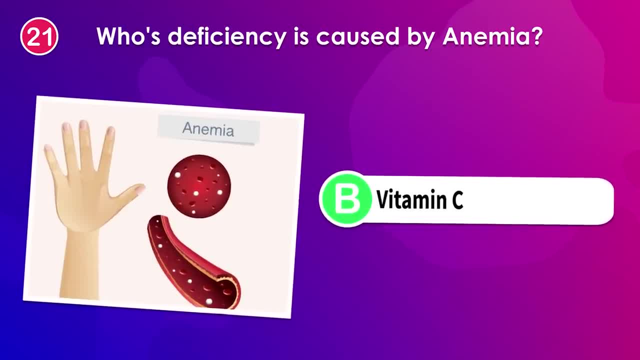 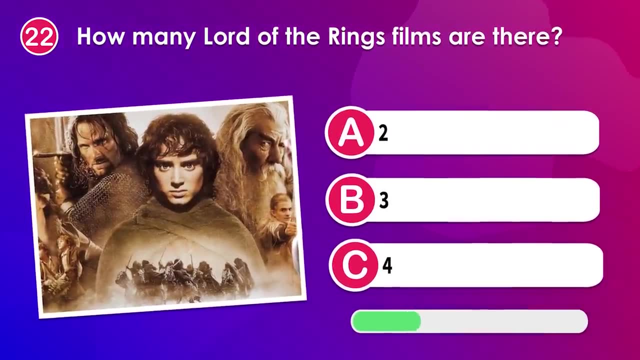 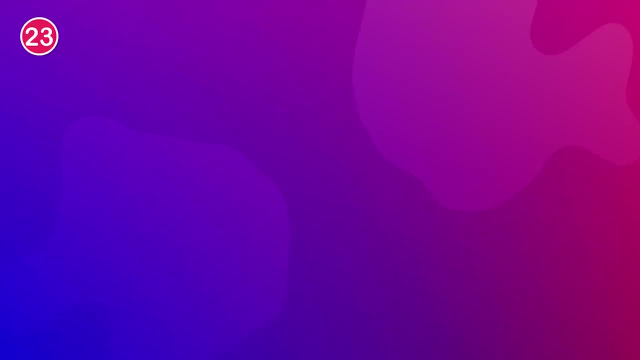 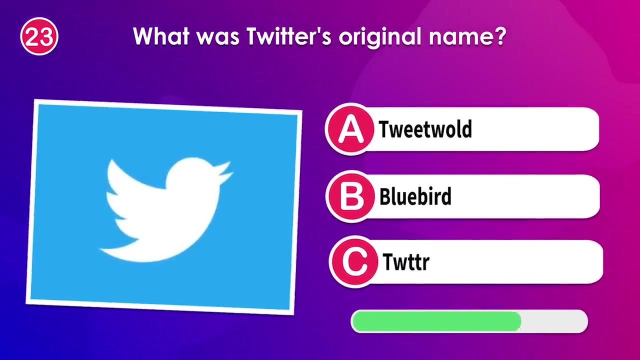 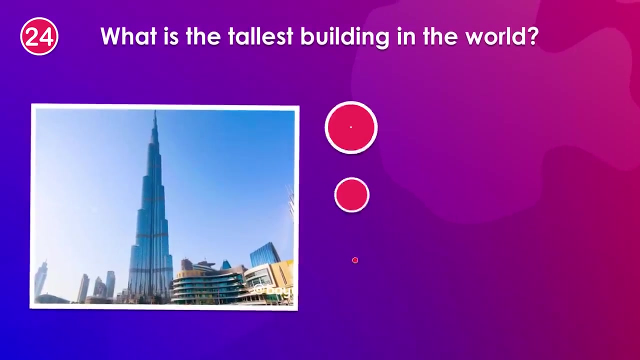 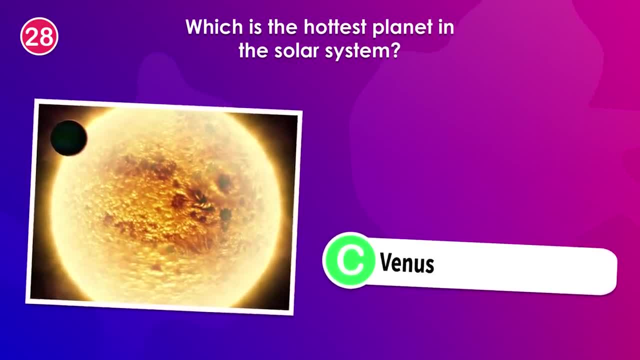 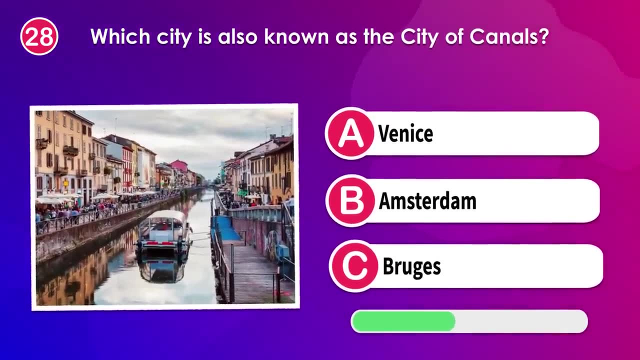 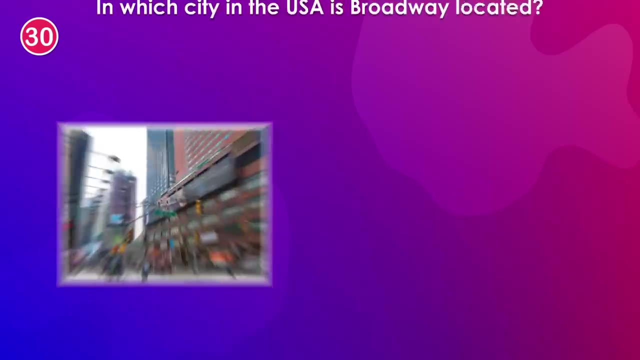 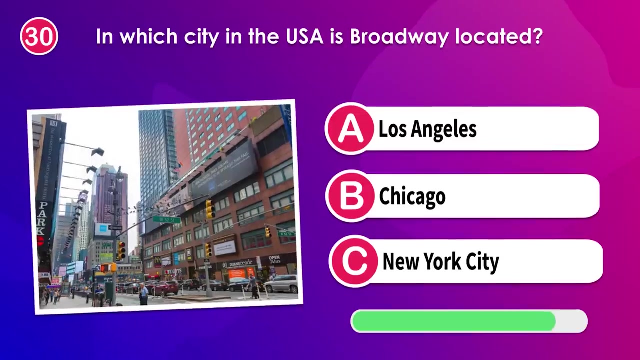 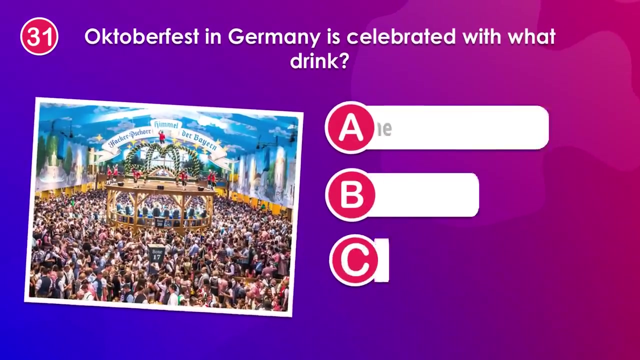 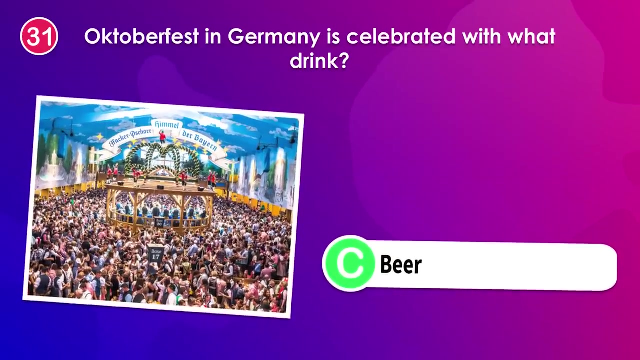 The answer is Venus. Which city is also known as the City of Canals? Yes, it's Venice. In which city in the USA is Broadway located? Octoberfest in Germany. Octoberfest in Germany is celebrated with what drink? Beer is the correct answer. 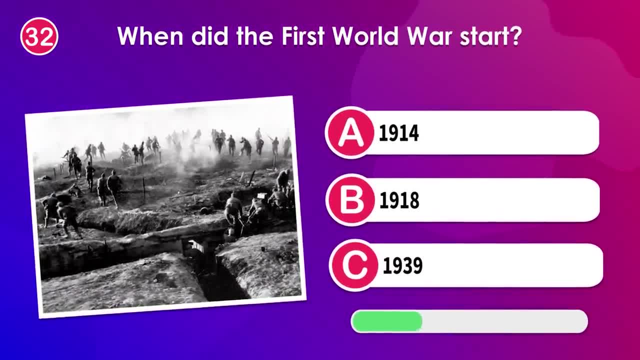 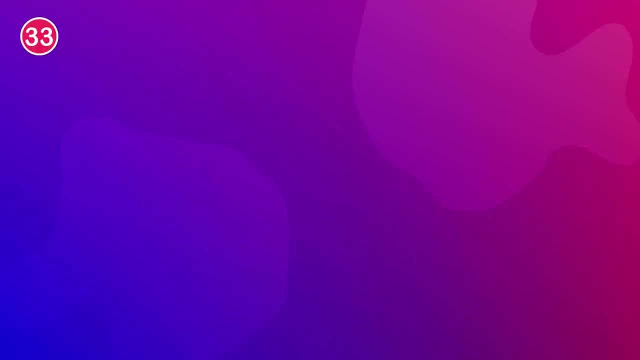 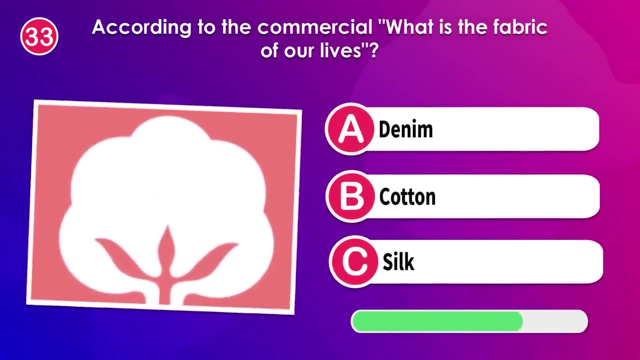 When did the First World War start? According to the commercial, what is the fabric of our lives? The answer is a book. The answer is a book. The answer is a book 6. Who is theLAN in New Zealand? 7.. 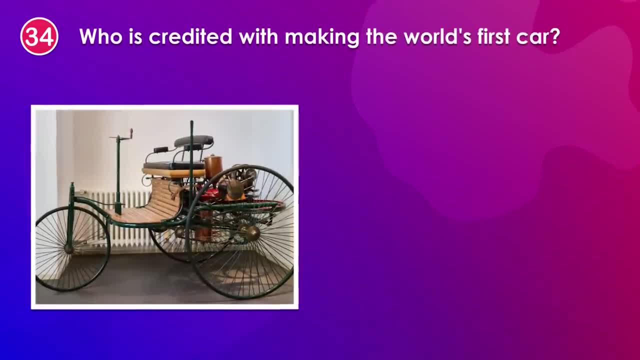 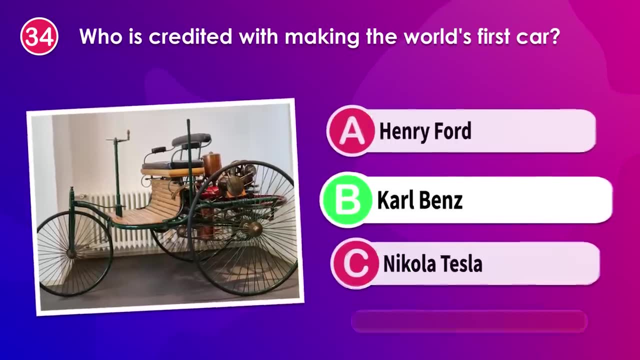 What is the color of the world? Yellow. What color is the moon in the world? Black, Black, Black. 7. Who is credited with making the world's first car? The answer is Portugal. 8. Who was the ancestor of the car? 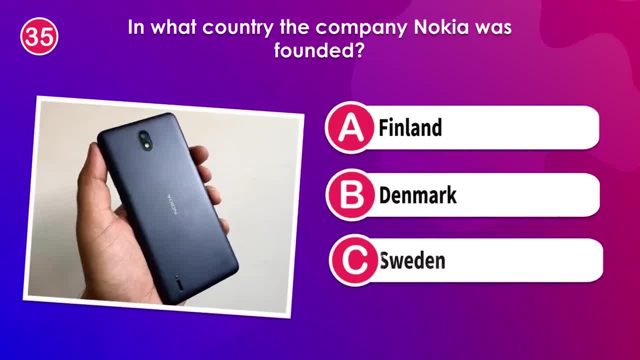 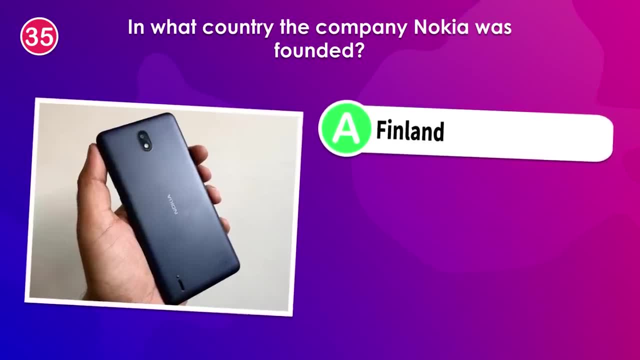 9. Who is credited with making the world's first car? 10. Who is credited with making the world's first car? 10. Carl Benz. 11. In what country the company Nokia was founded? 12. Who is known as the father of seasoning? 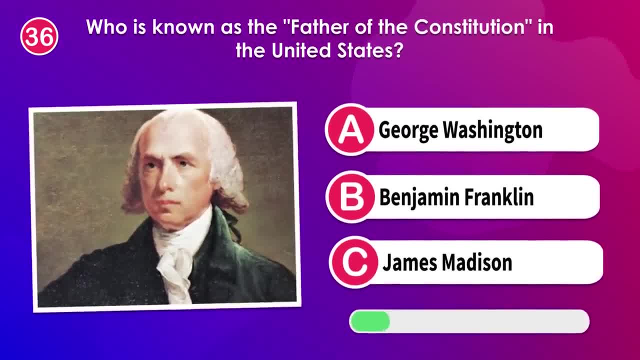 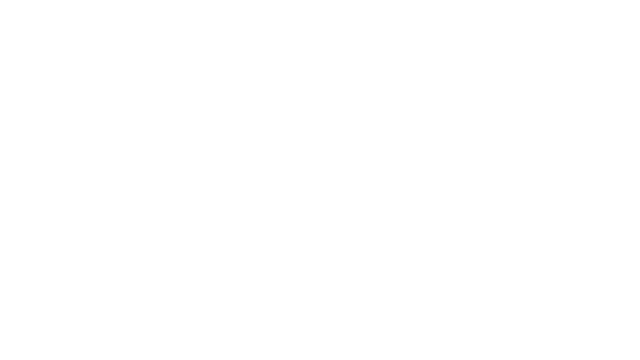 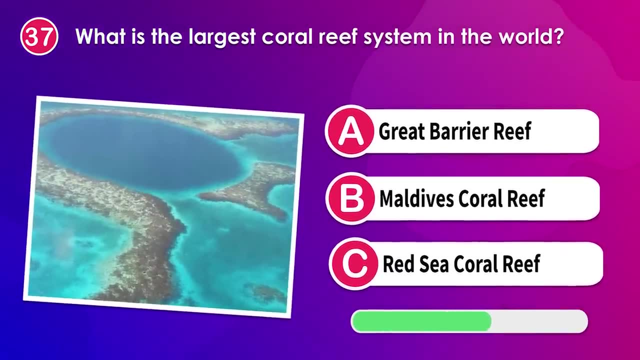 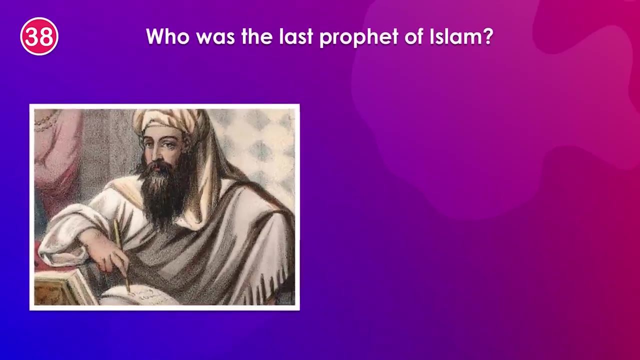 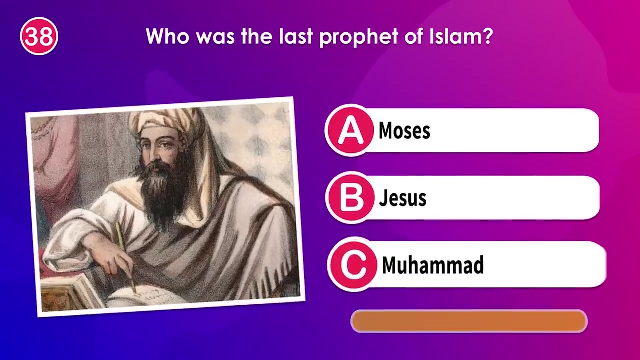 13., 12. 15., 14., 16., 16., 17., 17. 16. of the Constitution in the United States? yes, it is James Madison. what is the largest coral reef system in the world? who was the last prophet of Islam? the correct answer is: Muhammad. which country? 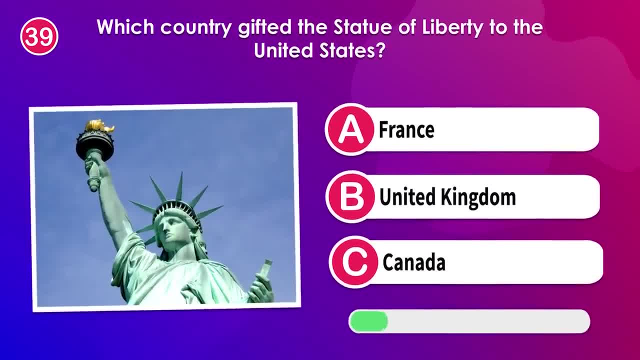 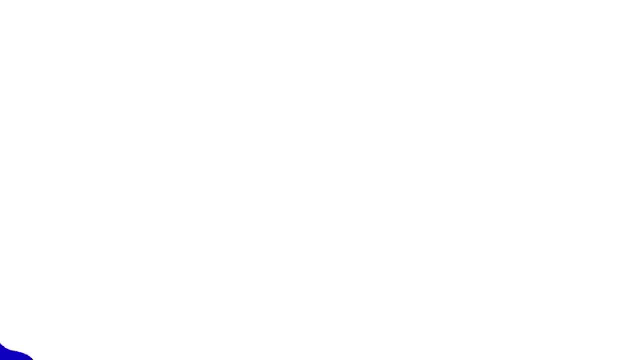 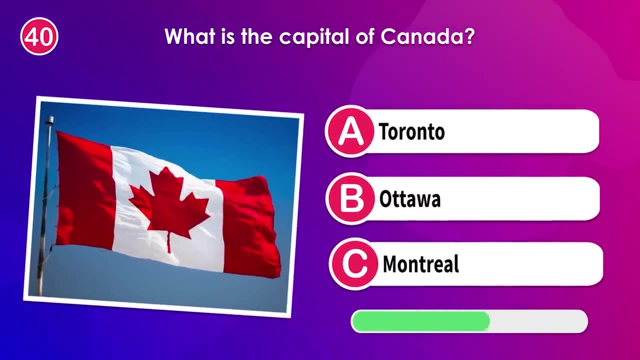 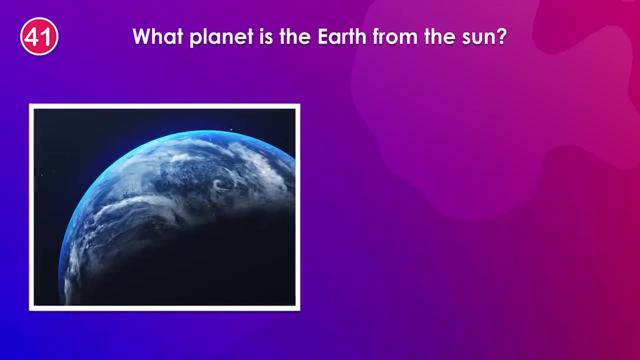 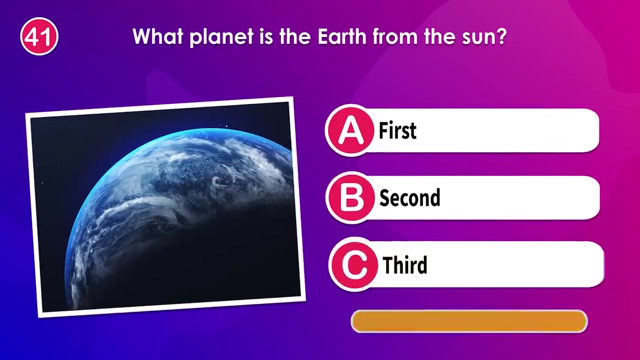 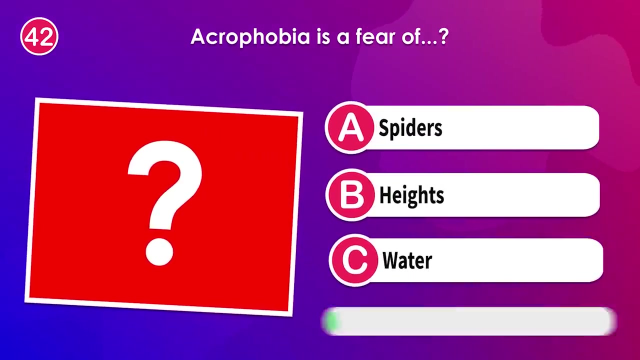 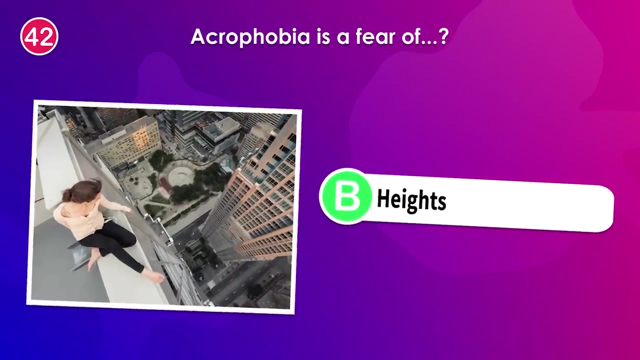 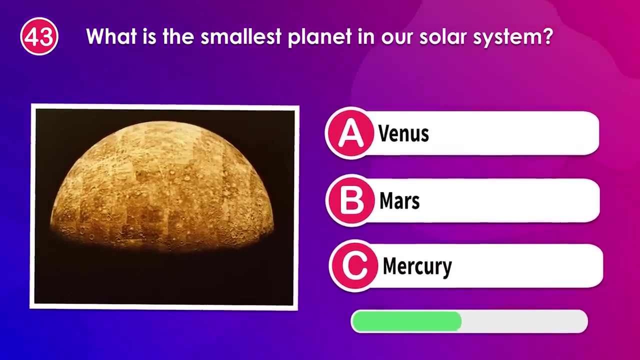 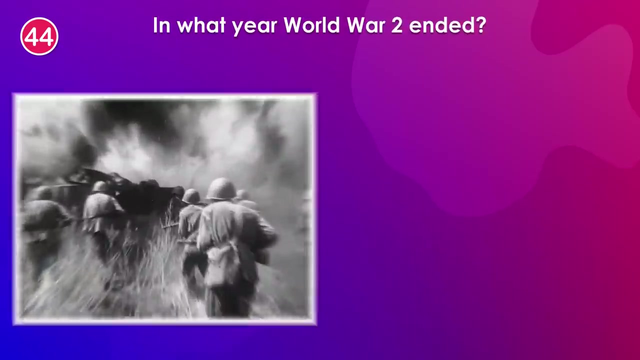 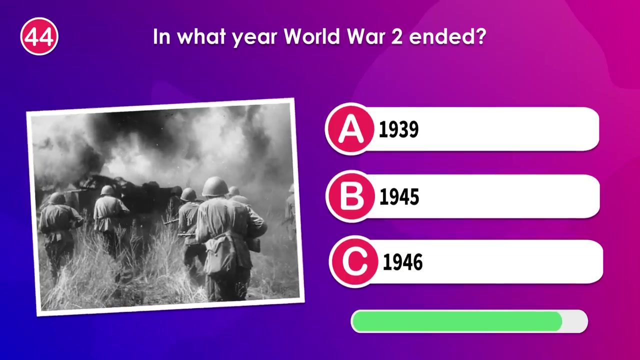 gifted the Statue of Liberty to the United States. what is the capital of Canada? it's Ottawa. what planet is the earth from the Sun? acrophobia is a fear of today's. what is the smallest planet in our solar system? the correct answer is mercury, in what your world war two ended. 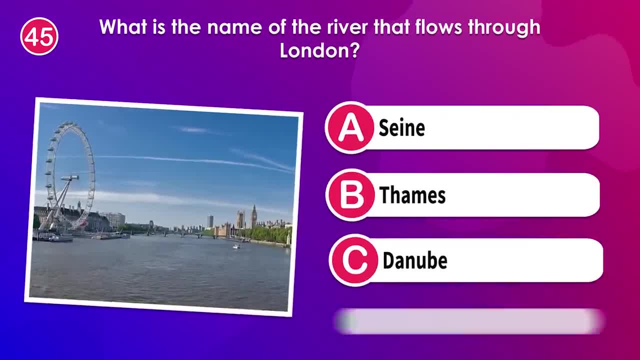 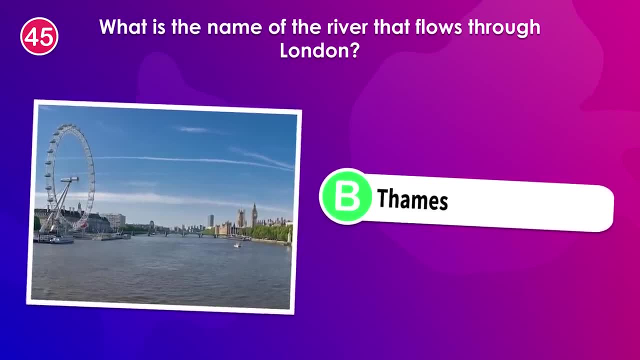 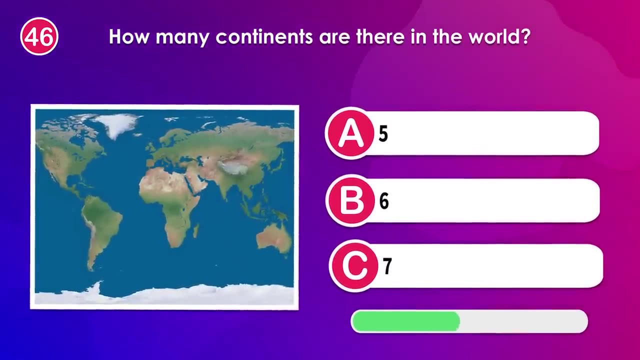 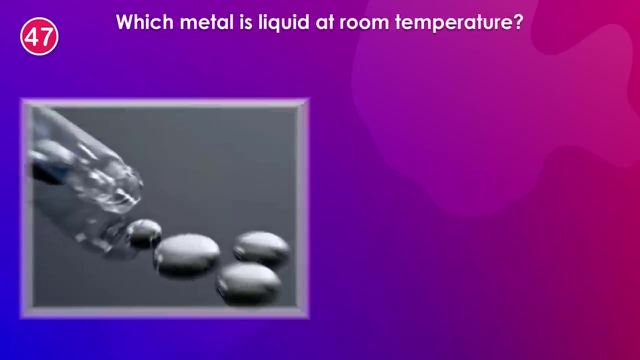 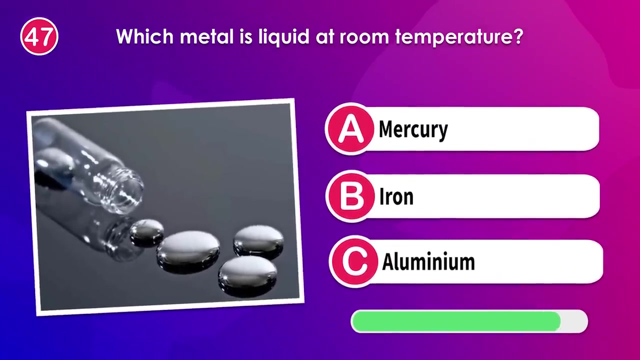 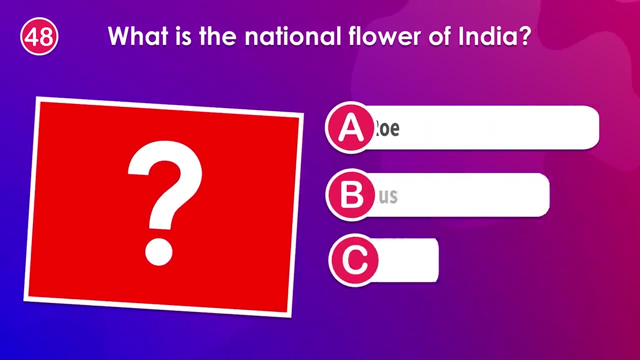 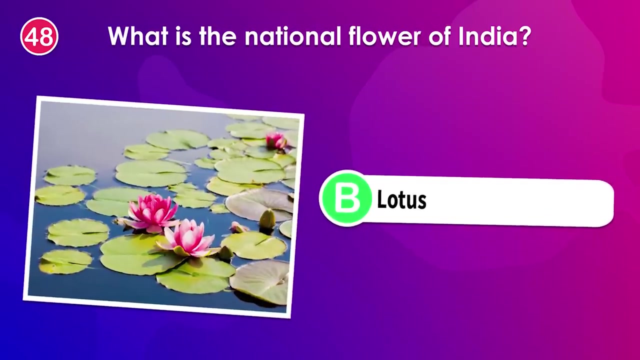 What is the name of the river that flows through London? How many continents are there in the world? The correct answer is seven. Which metal is liquid at room temperature? It's mercury. What is the national flower of India? Which chess piece can only move diagonally? 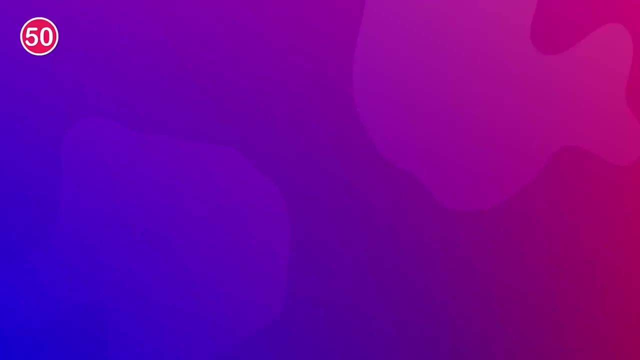 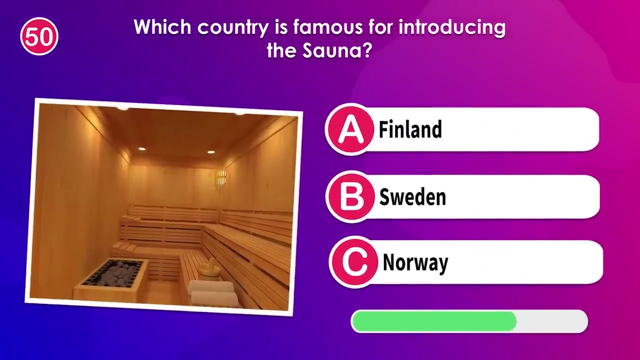 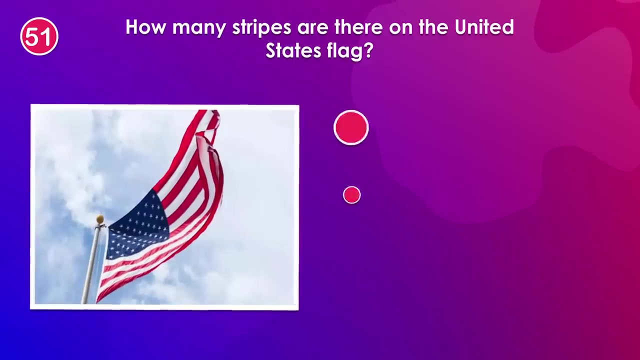 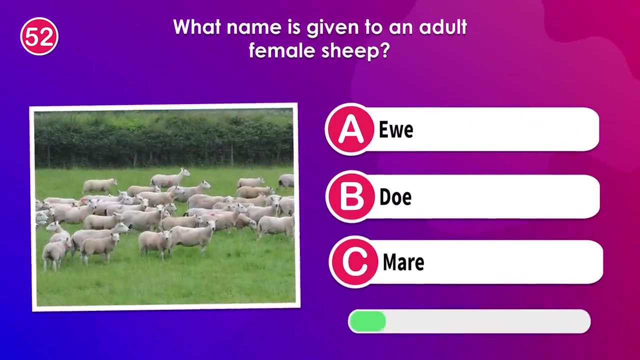 Yep, it's bishop. Which country is the most important? This country is famous for introducing the sauna. How many stripes are there on the United States flag? There are 13.. What name is given to an adult female sheep? It's close. 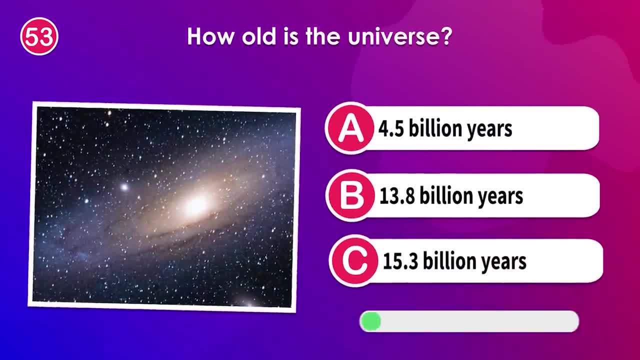 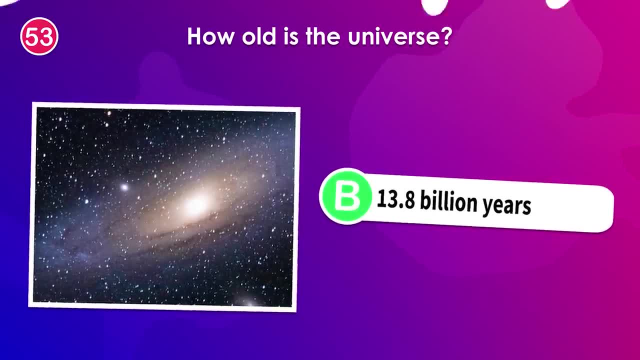 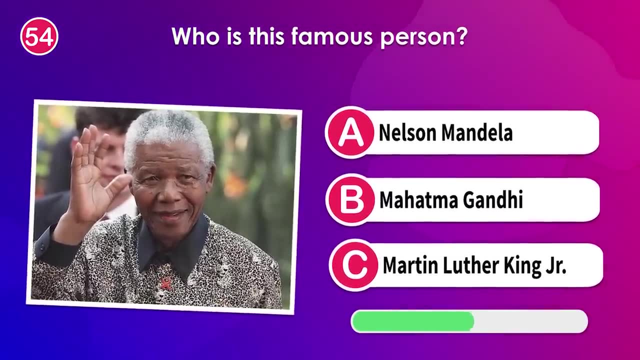 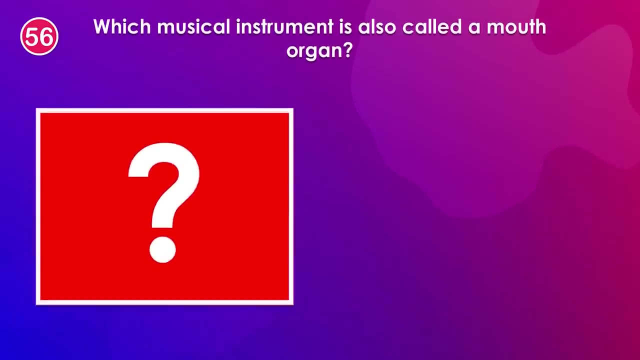 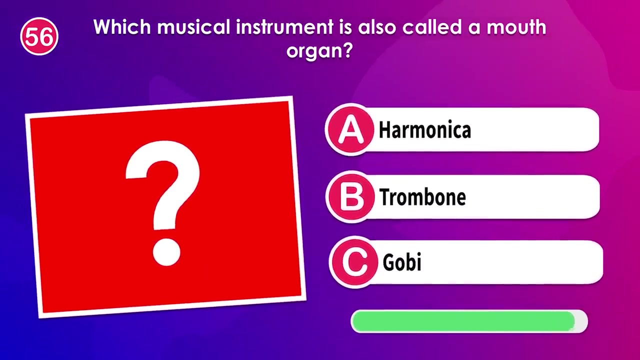 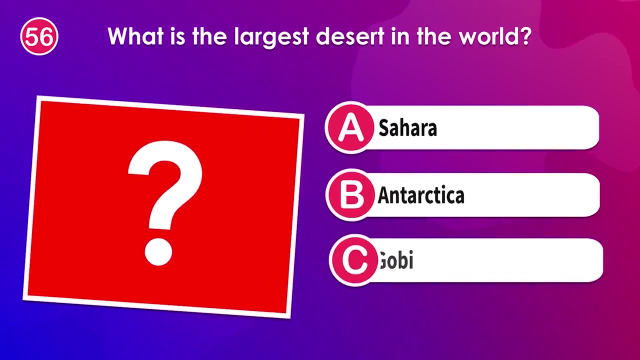 How old is the universe? Who is this famous person? This is Nelson Mandela. What is an instrument? What's the name of the musical instrument? Which musical instrument? Which musical instrument is also called a mouth organ? What is the largest desert in the world? 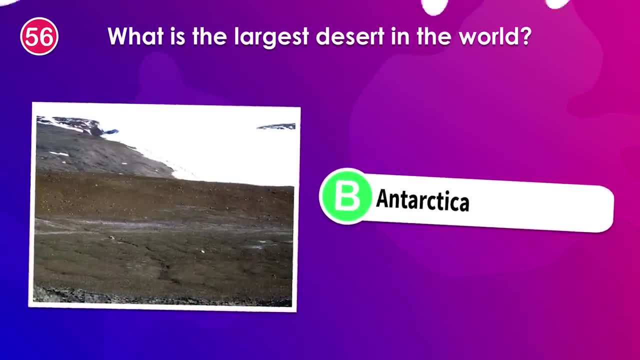 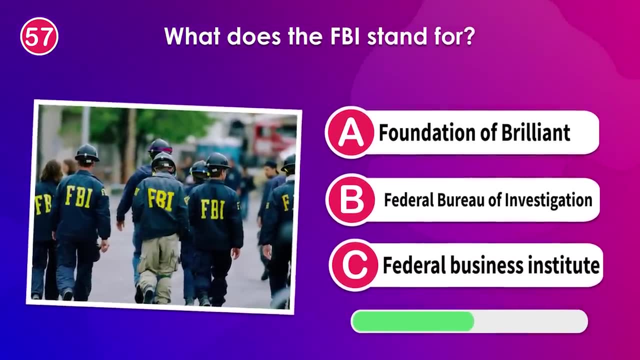 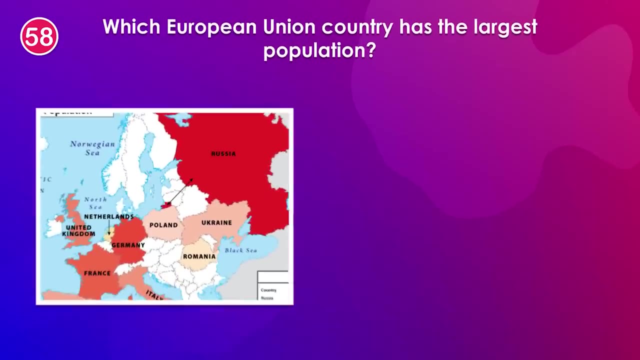 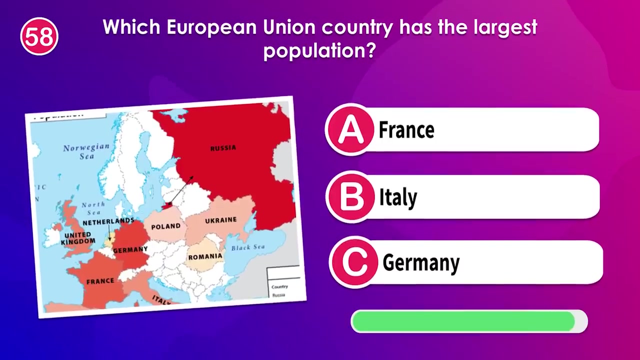 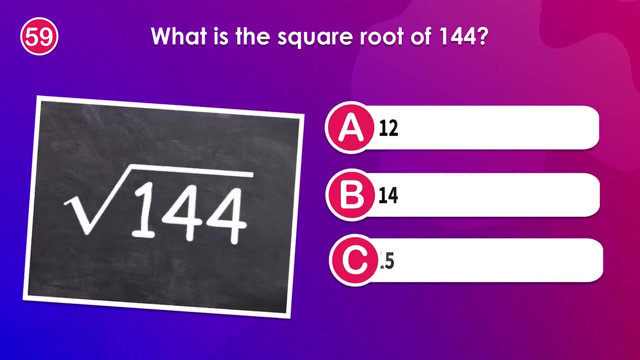 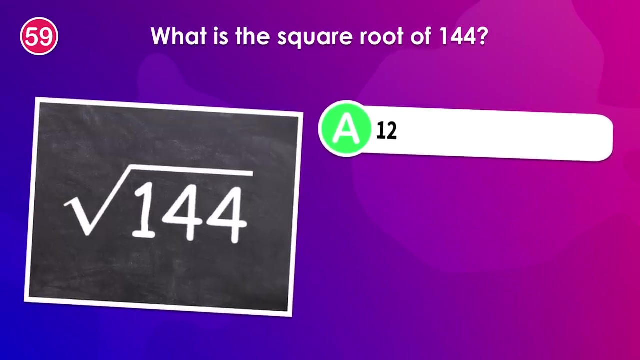 The correct answer is the Antarctic Polar Desert. What does the FBI stand for? Which European Union country has the largest population? It's Germany. What is the square root of 144?? Which country is the largest? China is the largest producer of tea. 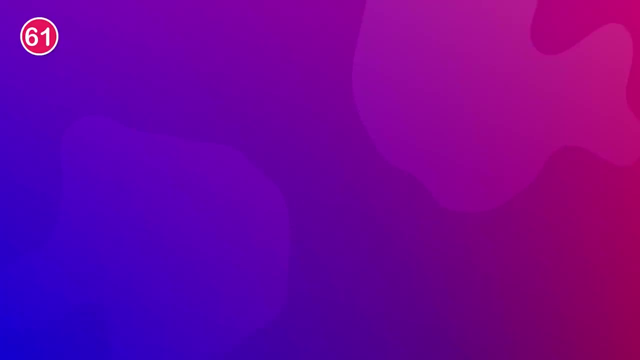 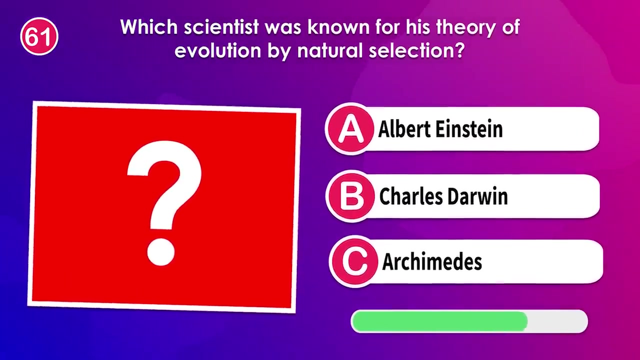 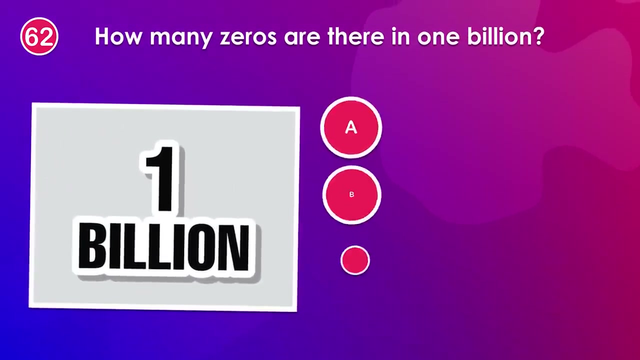 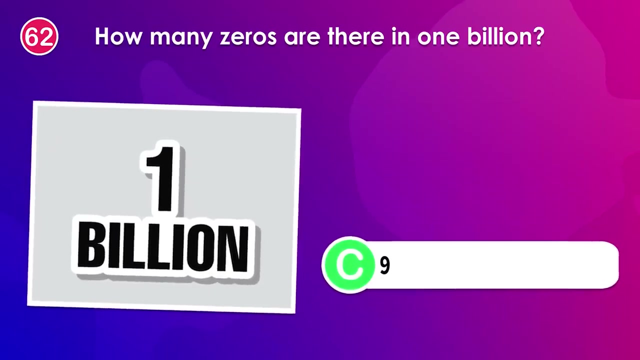 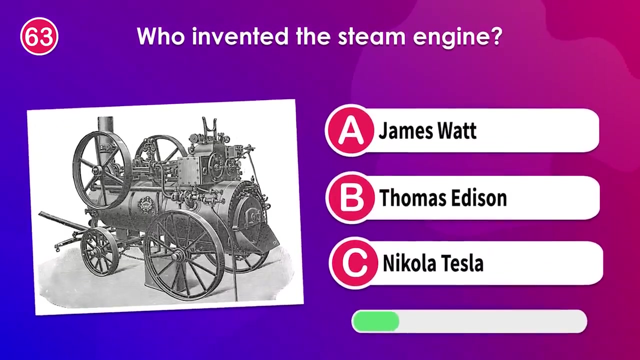 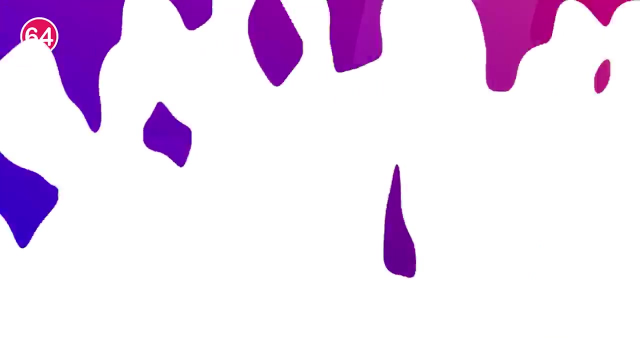 China is the right answer. Which scientist was known for his theory of evolution by natural selection? How many zeros are there in 1 billion? Who invented the steam engine? Who invented the steam engine? Who invented the steam engine? James Watt? From which movie is this famous quote? 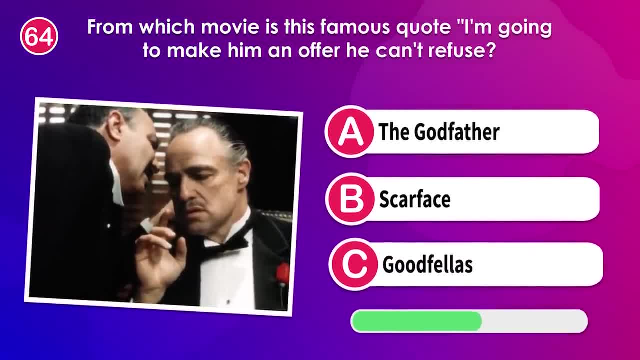 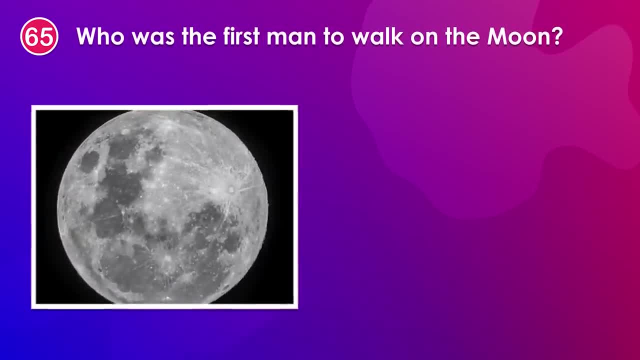 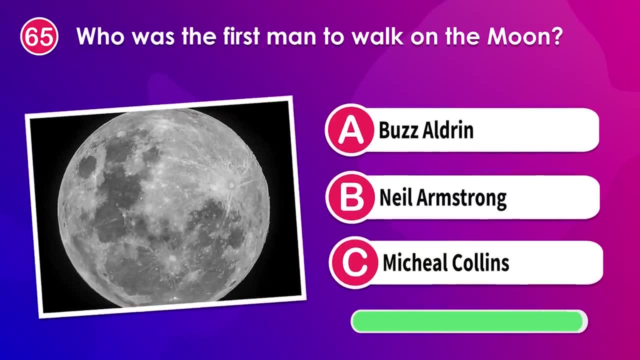 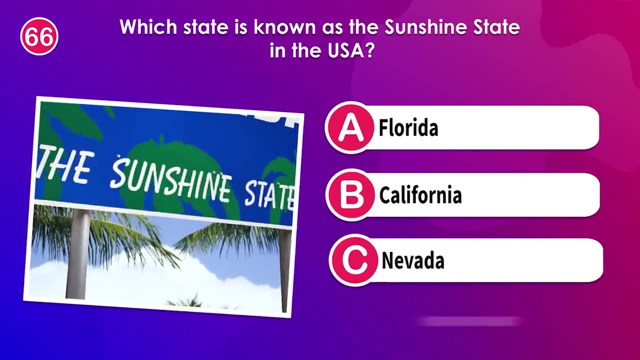 I'm going to make him an offer he can't refuse. The correct answer is The Godfather Who was the first man to walk on the moon. Is this a space surgery? Which state is known as the sunshine state in the USA? You are right, Canada is the most startling country in the world. 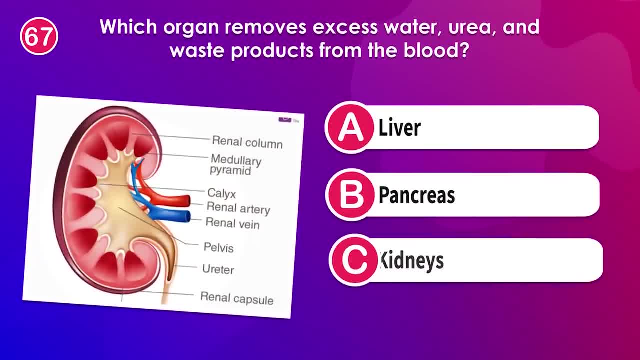 Which organ removes excess water, urea and waste products from the blood? It's the aspirean��kd, or favorable liver function. Which 부분 of the cell? the liversized? It's the cervical. It's the cervical Right. 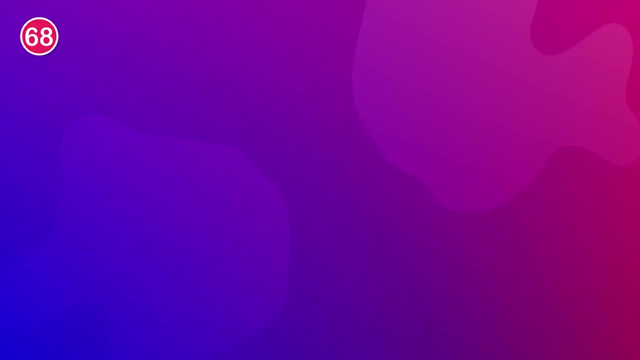 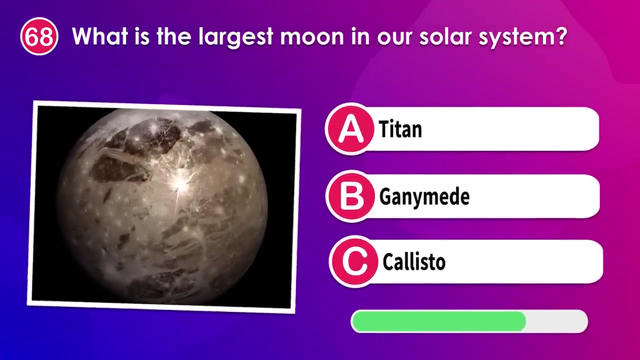 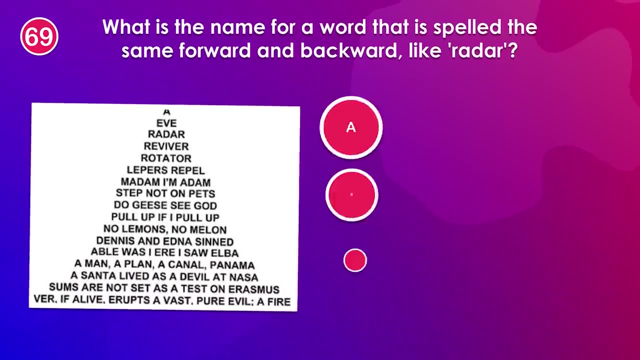 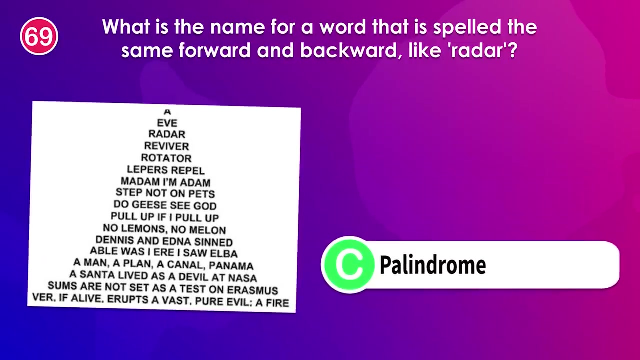 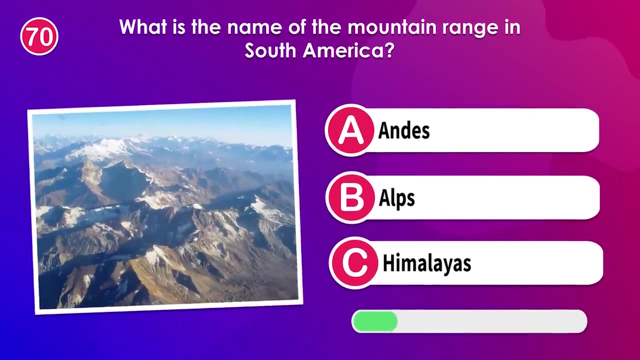 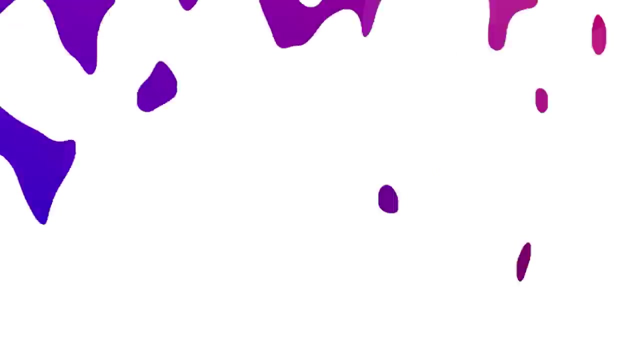 It's the cervical. The correct answer is kidney. What is the largest moon in our solar system? What is the name for a word that is spelled the same forward and backward, like radar? It is called palindrome. What is the name of the mountain range in South America? 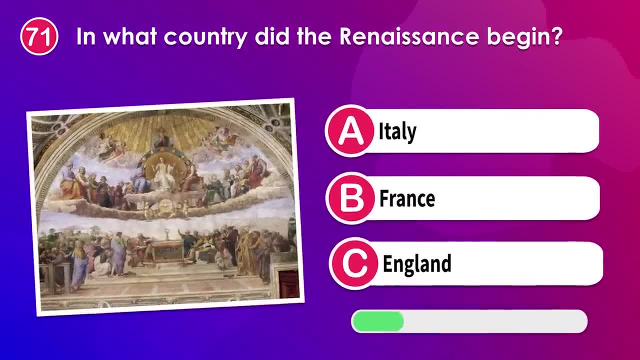 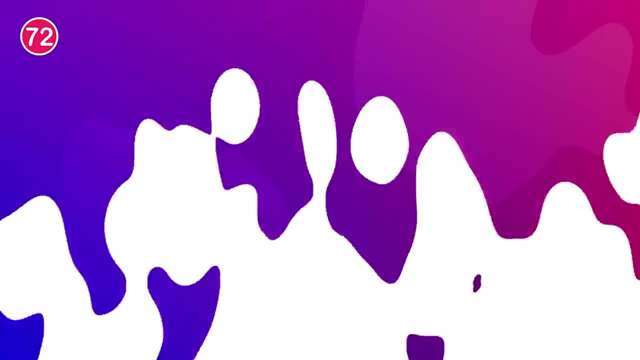 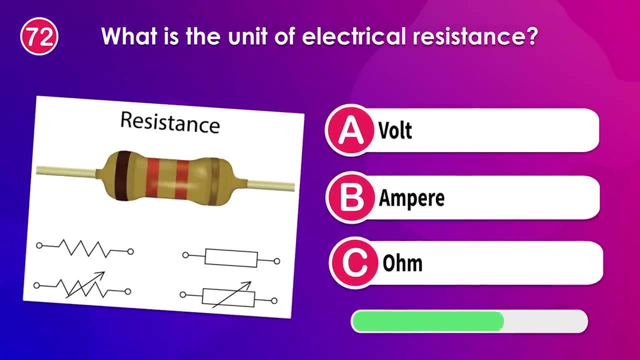 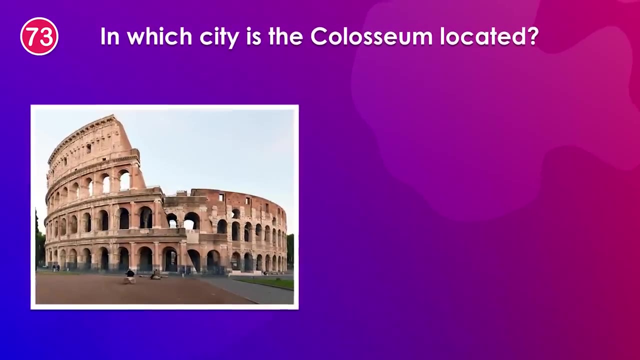 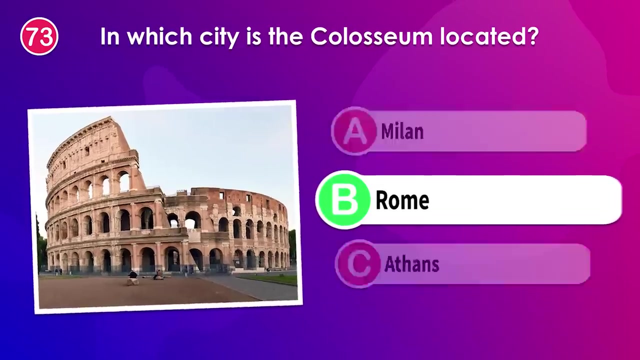 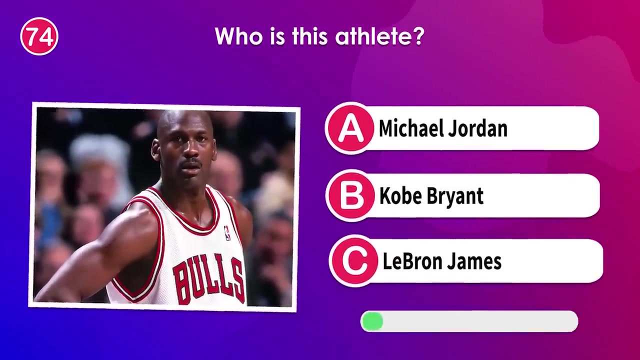 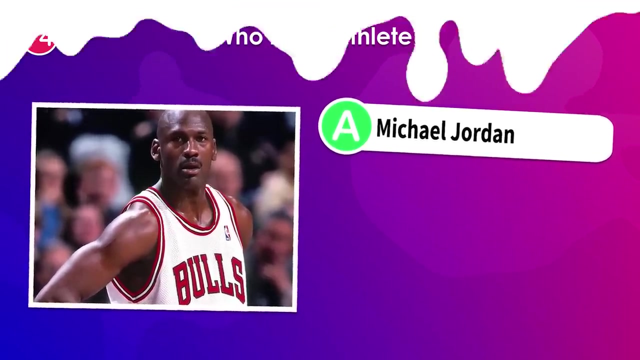 In what country did the renaissance begin? What is the unit of electrical resistance? It is called a motor. In which city is the Colosseum located? Yes, it's Rome. Who is this athlete? He is the famous Michael Jordan. 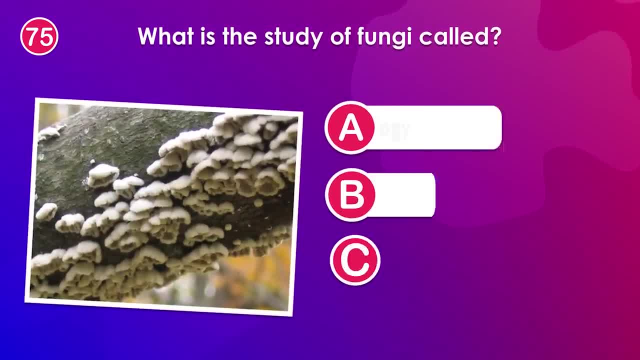 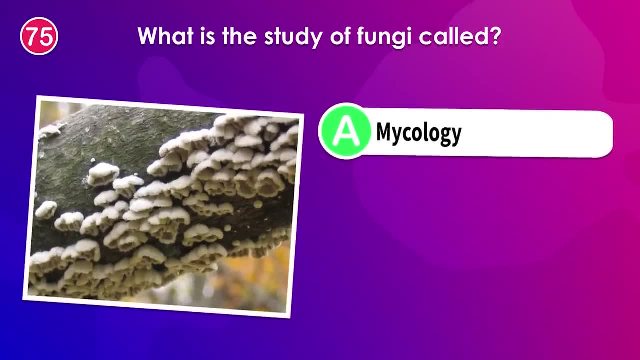 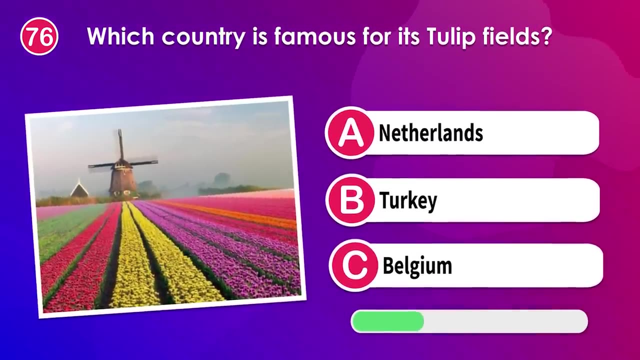 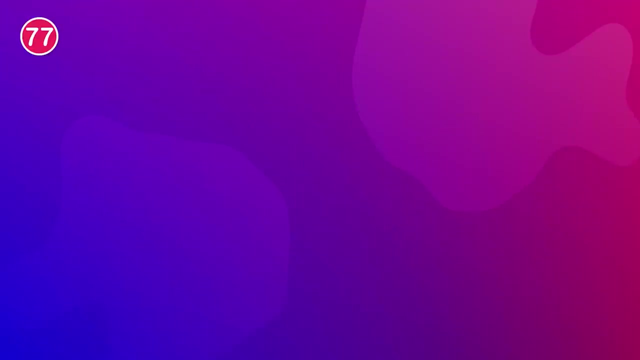 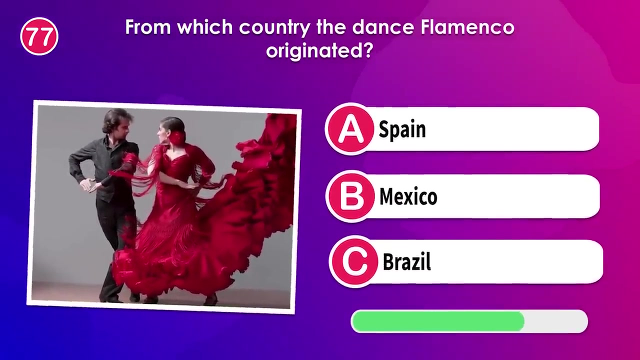 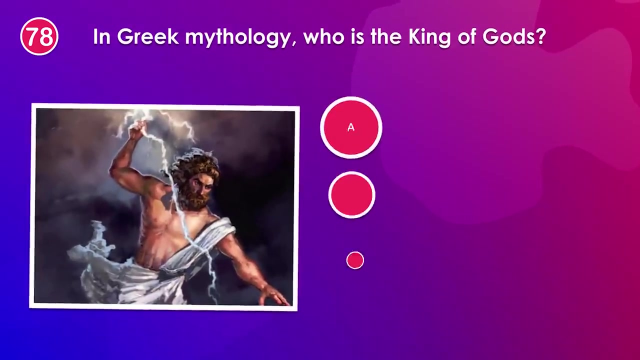 What is the name of the planet Rome? What is the study of fungi called? Which country is famous for its tulip fields? From which country the dance flamenco originated? France, France, France. The correct answer is Spain. In Greek mythology, who is the King of the Gods? 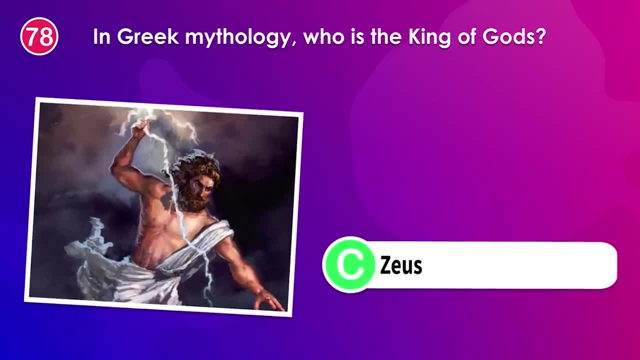 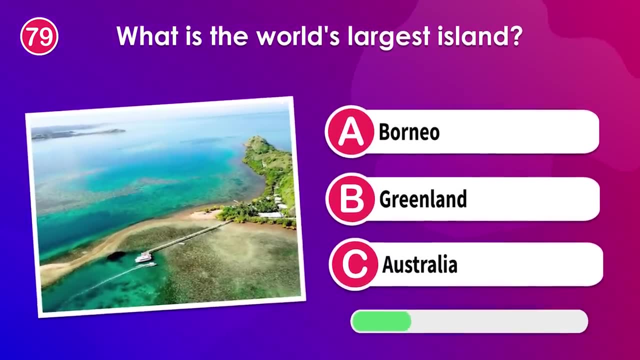 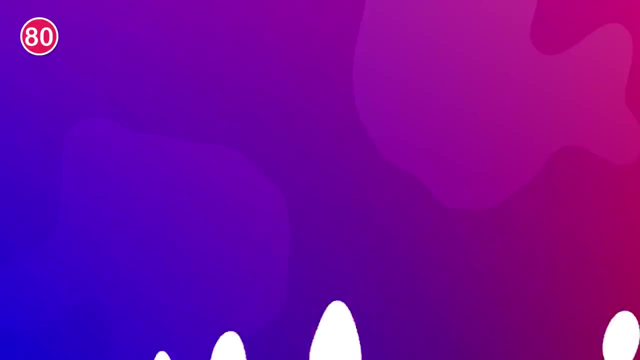 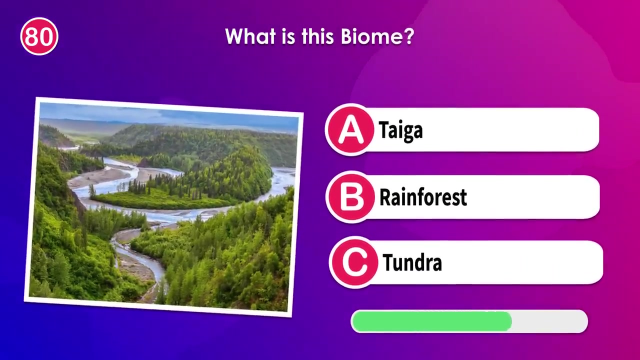 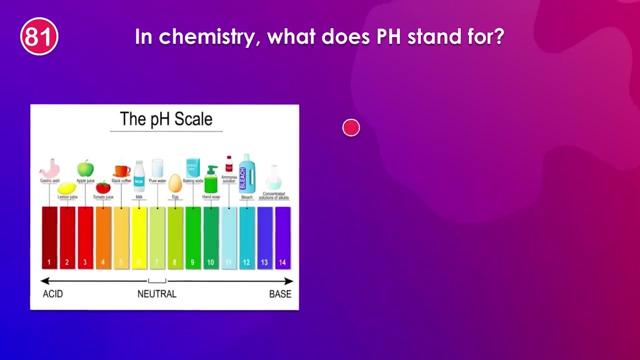 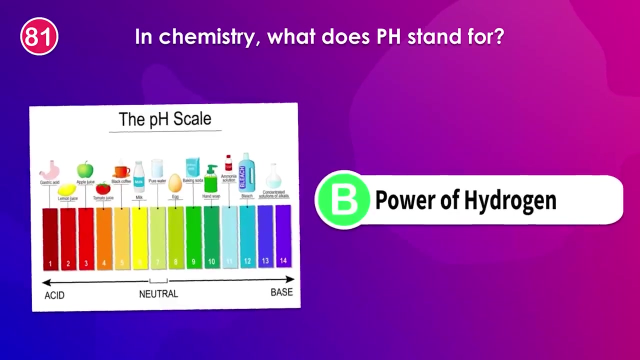 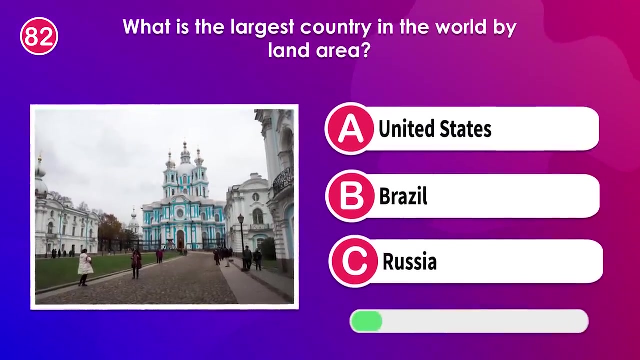 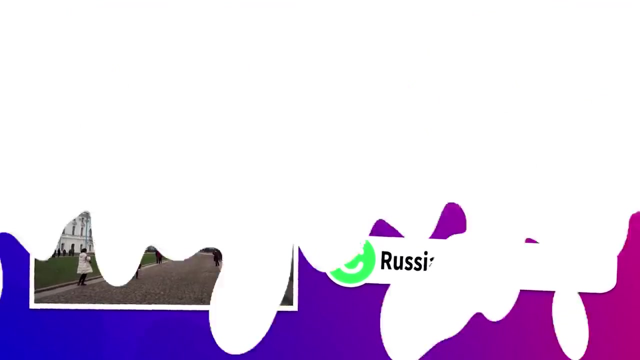 It's Zeus. What is the world's largest island? The answer is Greece. What is this biome? The answer is taiga. In chemistry, what does pH stand for? What is the largest country in the world by land area? What is the sum of the angles in a triangle? 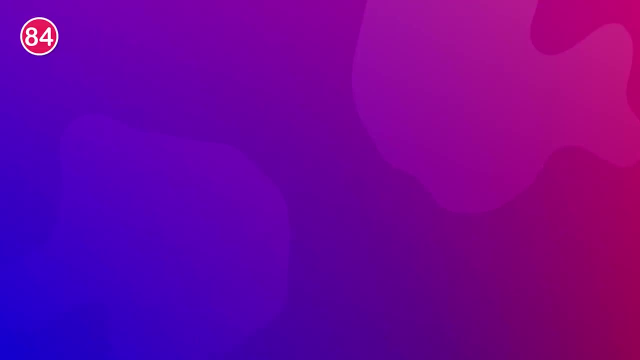 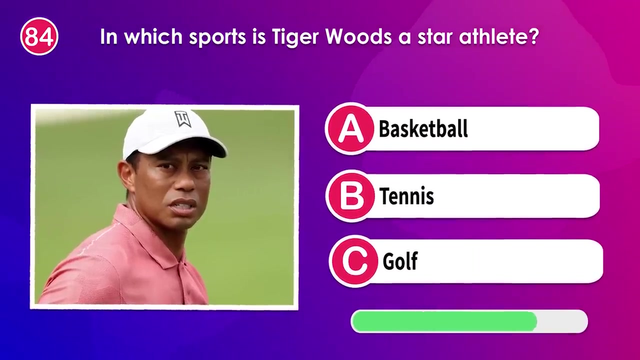 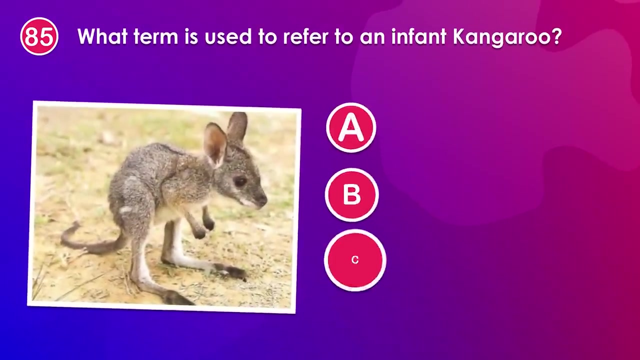 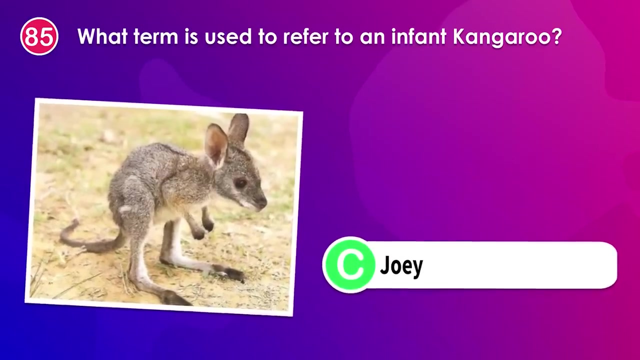 180 degrees, In which sports is Tiger Woods a star athlete? What is the largest city in the world by land area? This term is used to refer to an infant kangaroo. It's called Joey. What was the first successful vaccine developed for? 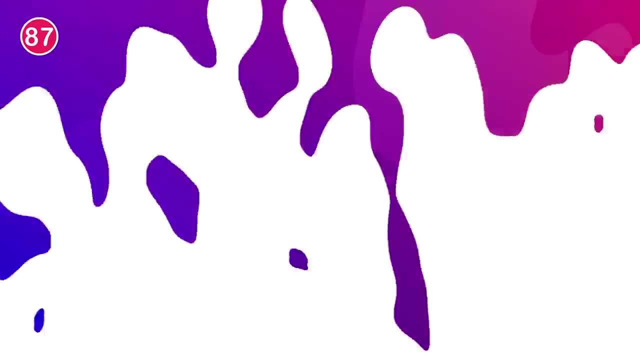 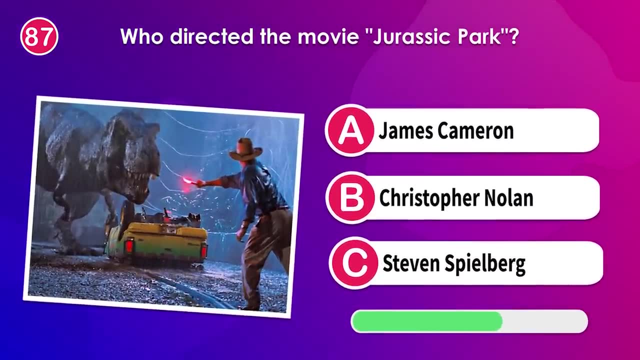 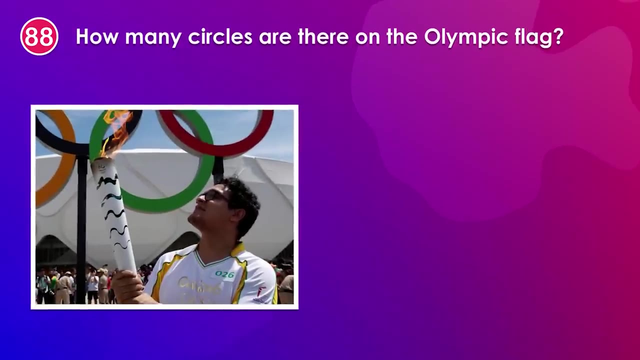 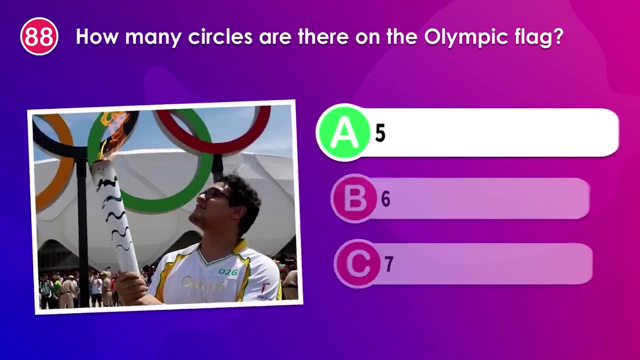 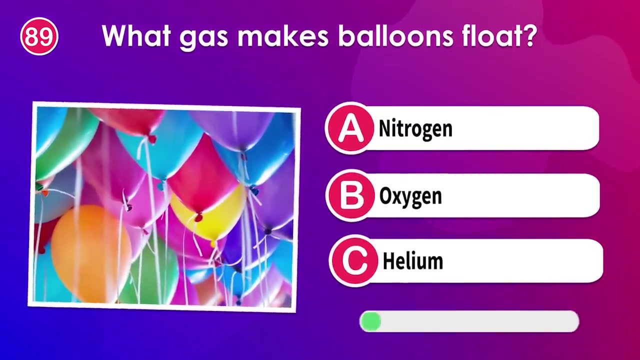 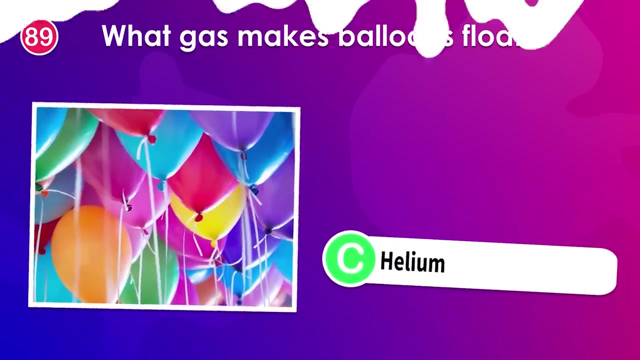 It was for smallpox, Who directed the movie Jurassic Park, Thailand. How many circles are there on the Olympic flag? There are five. What gas makes balloons float? The correct answer is helium. What is its number? 13-13Kg-8.. 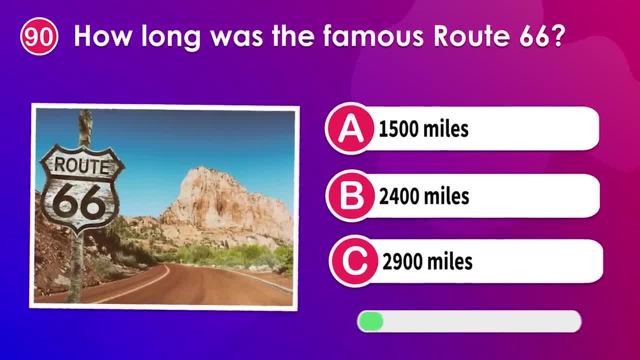 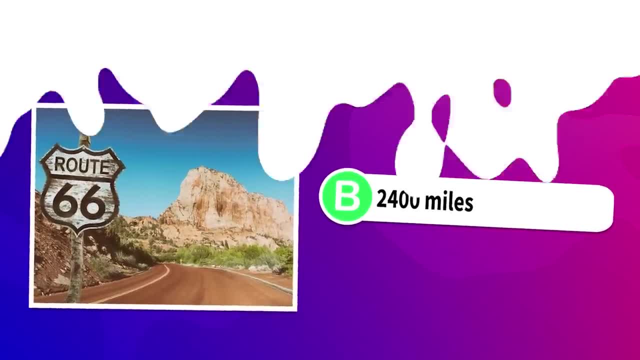 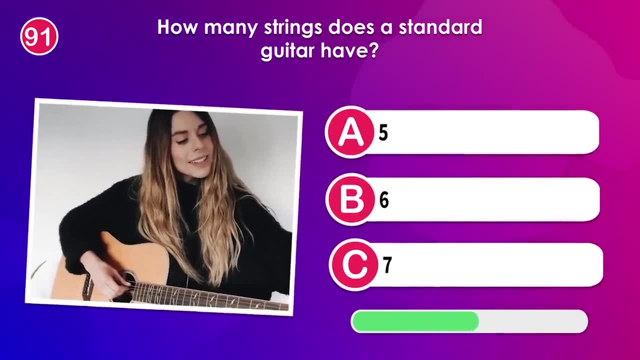 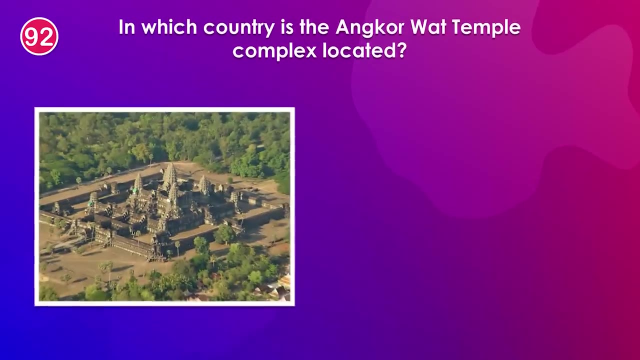 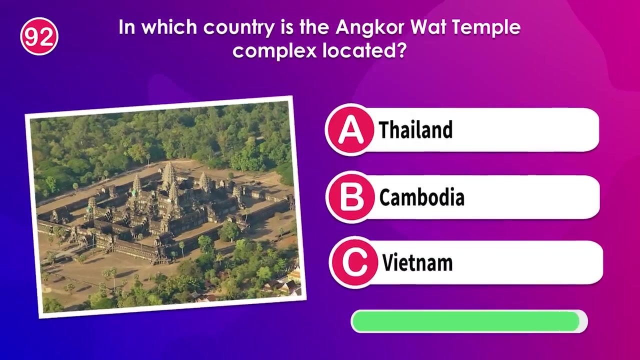 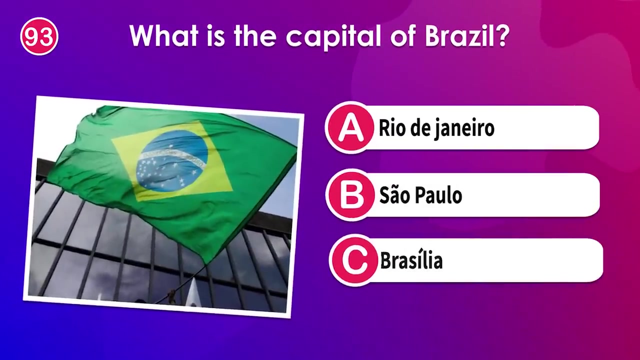 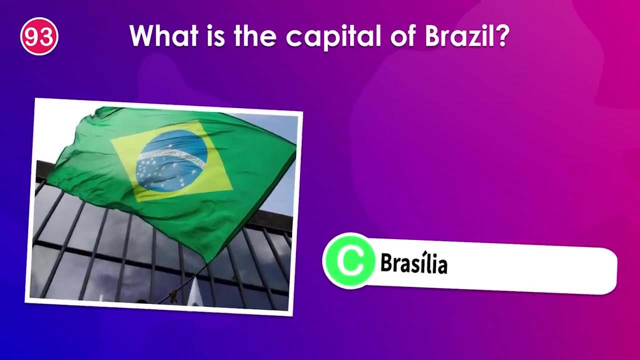 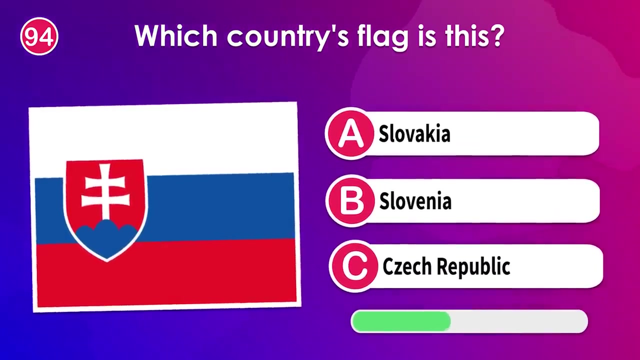 One input. What was the famous Route 66?? How many strings does a standard guitar have? The correct answer is six. In which country is the Angkor Wat Temple Complex located? What is the capital of Brazil? It's Brasilia. Which country's flag is this?